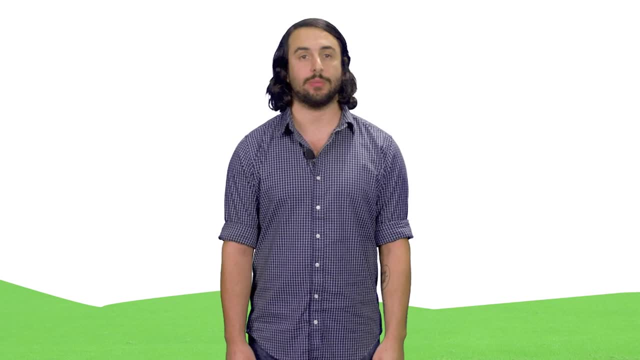 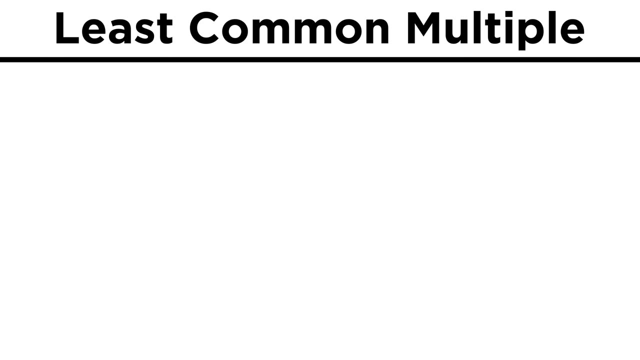 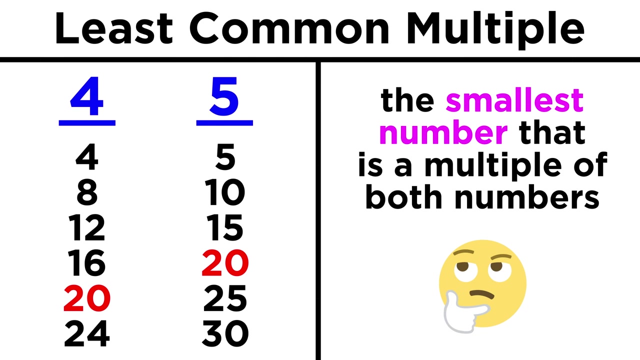 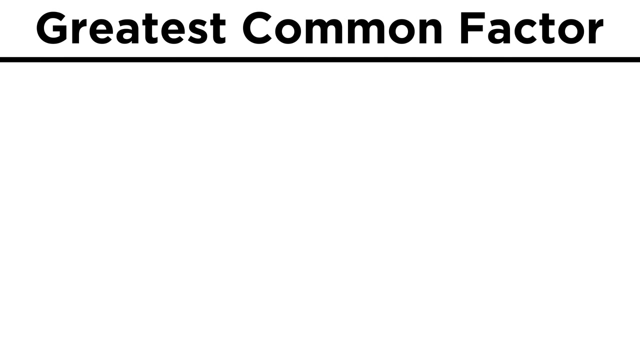 Professor Dave, again let's talk about greatest common factors. We just learned about least common multiples. These can be found when comparing two numbers and finding the smallest number, that is, a multiple of both of them. By the same token, we will want to be able to identify the greatest common factor of. 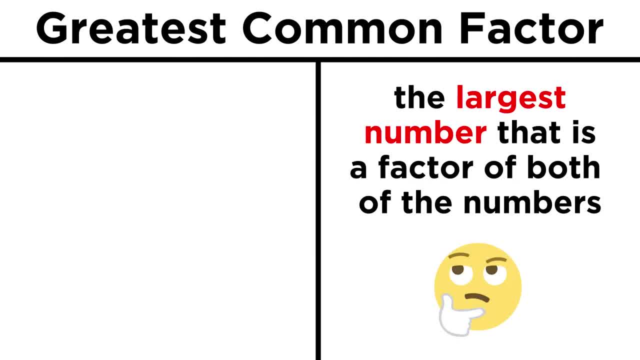 two numbers. As you might be able to guess, this is the largest number. that is a factor of both the numbers. Take, for example, ten and fifteen. If we write out all the factors for ten, that would be one, two, five and ten. 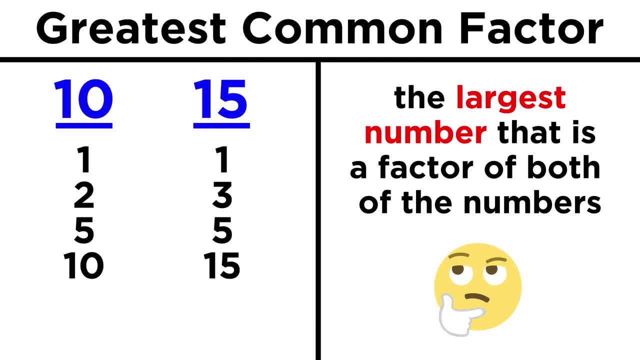 For fifteen, that would be one, three, five and fifteen. The largest number that can be found in both of these lists is five. so five is the greatest common factor of these two numbers. Now let's try eighteen and twenty-four. 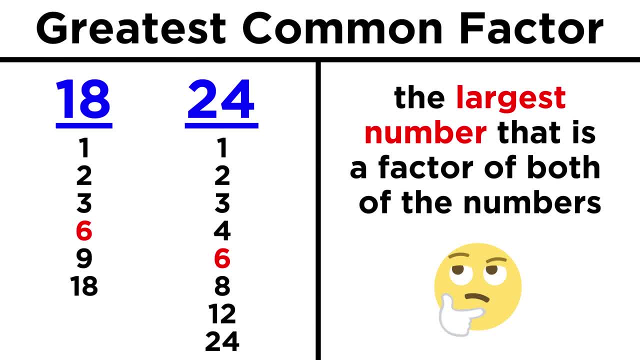 Here are all the factors for both of these numbers and we will find that six is the largest factor. that is common to both lists. So six is the greatest common factor of eighteen and twenty-four, Just like with the least common multiples. this is easy to do for small numbers because 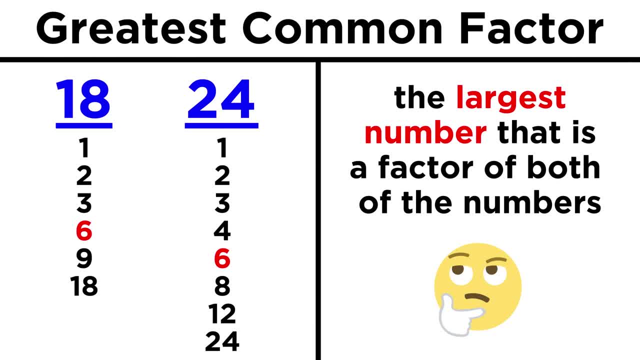 they will have only a handful of factors, so we can just list them all and compare. But again, as numbers get larger it may become more difficult to find the largest number, So let's try eighteen and twenty-four. Here are all the factors for both of these lists. Just like with the least common factors. this is easy to do for small numbers because they will have only a handful of factors, so we can just list them all and compare. But again, as numbers get larger it may become tedious to identify and list every single. 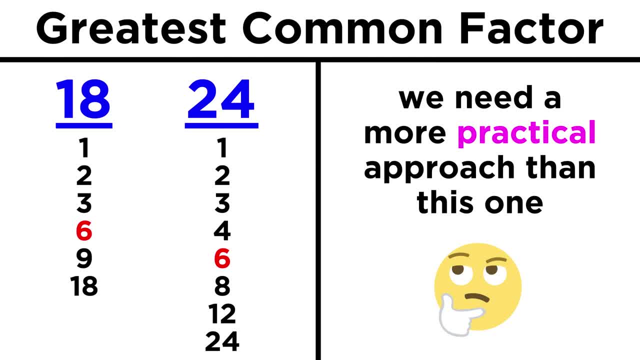 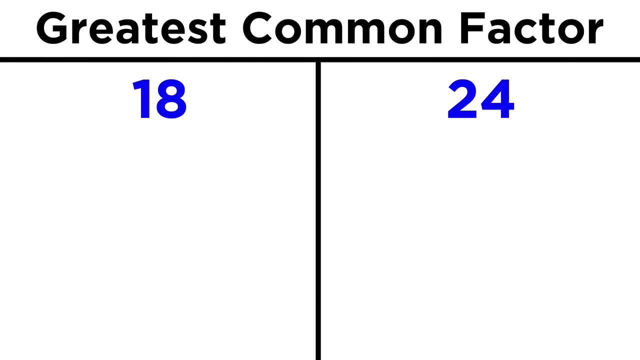 factor for a number. So there is a bit of a trick to this as well. Let's look at the same example we just did. We can carry out the prime factorization of both numbers, and that would give us two times three times three and two times two times two times three. 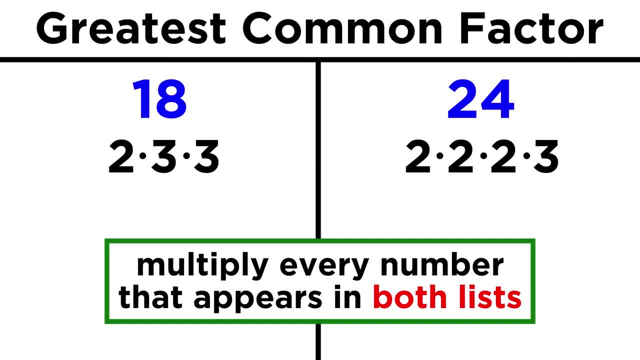 Once we have this, all we do is take all the numbers that appear in both lists as many times as they appear in both of them. And let's take the numbers that appear in both lists as many times as they appear in of the lists and multiply them together. 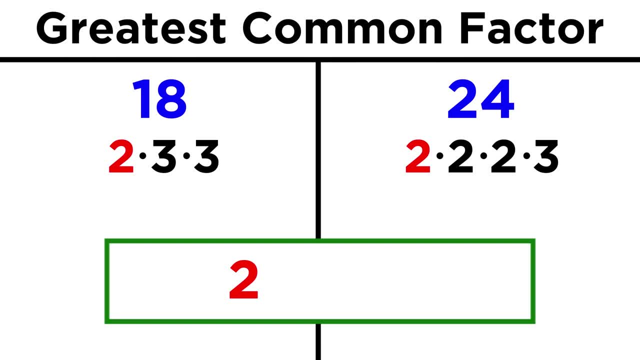 So this first two, that's in both, so let's pull that aside. This three, that's also in both, so let's pull that aside as well. Now we are done, because one list has a three left and no twos and the other list has. 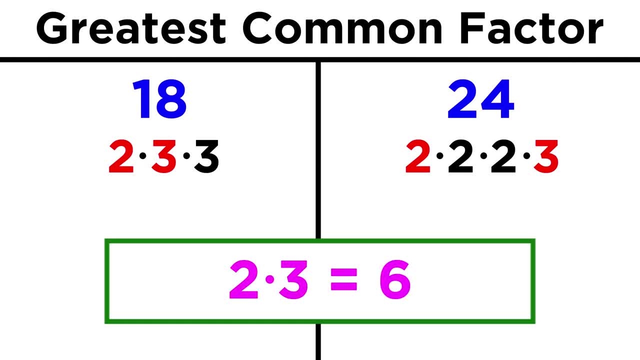 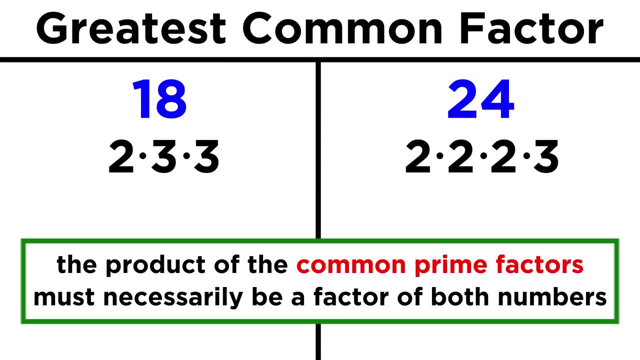 some twos but no threes. Now we take the two and three, we pulled aside and multiply them together to get six, which we already knew was the answer. This works because if we take all of the prime factors present in both lists, they must necessarily 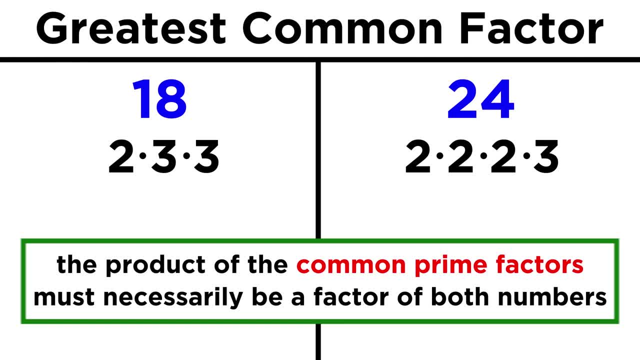 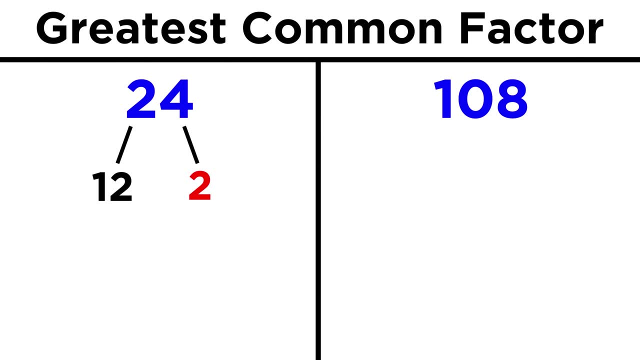 give a product that is a factor of both numbers and with no more prime factors left in common. to multiply, this will necessarily be the greatest common factor. Let's try the same thing for twenty-four and a hundred and eight For twenty-four. let's chop that up into twelve times two, the twelve into four times. 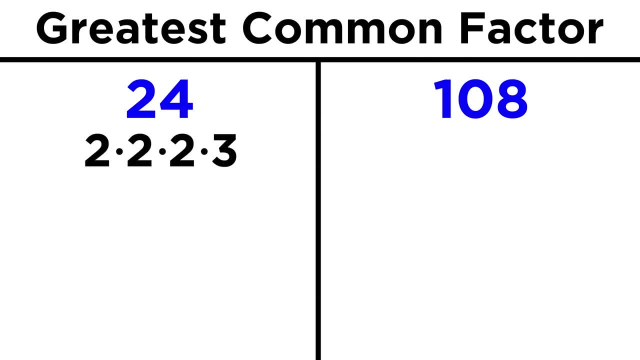 three And the four into two times two. That gives us two times two times two times three, For a hundred and eight. let's cut it in half, Cut the fifty-four in half, cut the twenty-seven into three and nine and nine into three and 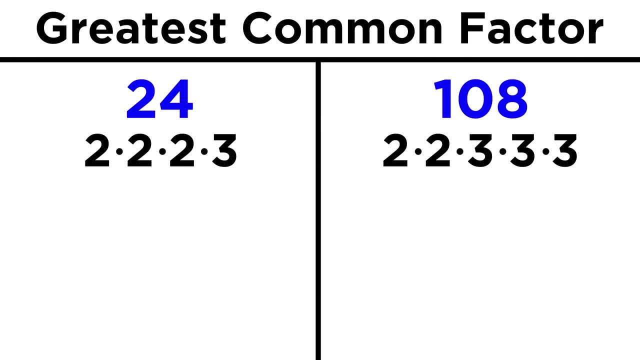 three. That gives us two times two times three times three times three. Now we see what we have in both lists. We take one of the twos, another two and a three, and that's all we can do. so two times two. 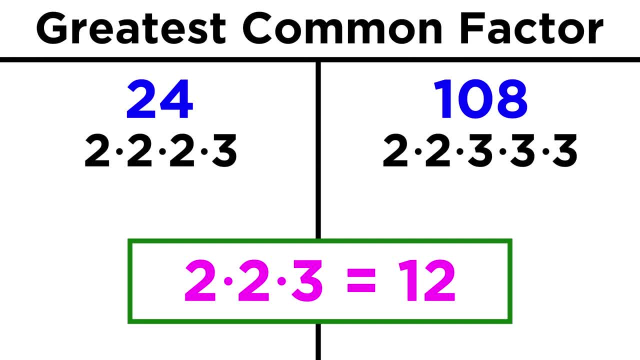 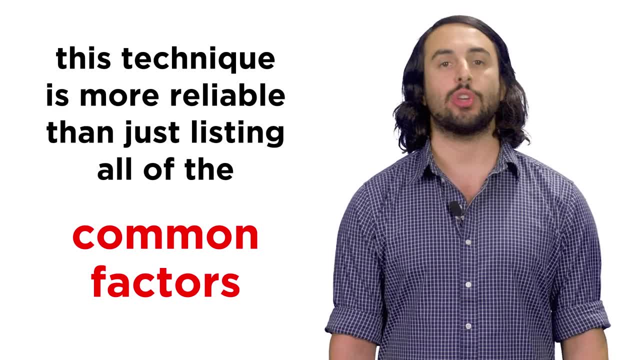 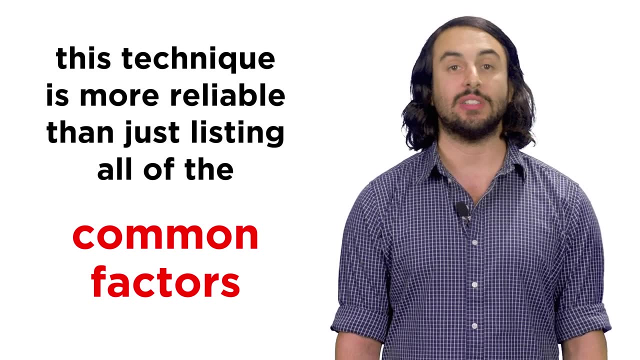 times three is twelve, and that's the greatest common factor for these two numbers. This technique is reliable, no matter how big the numbers get, so it eventually becomes a much better strategy than listing all the factors and examining the lists. Let's check comprehension. 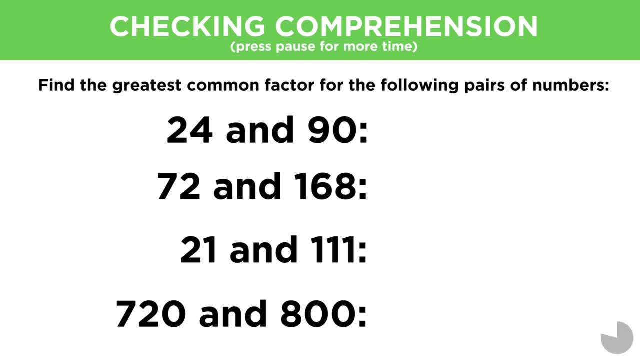 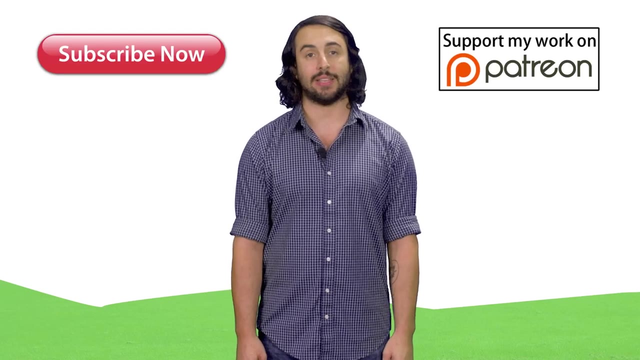 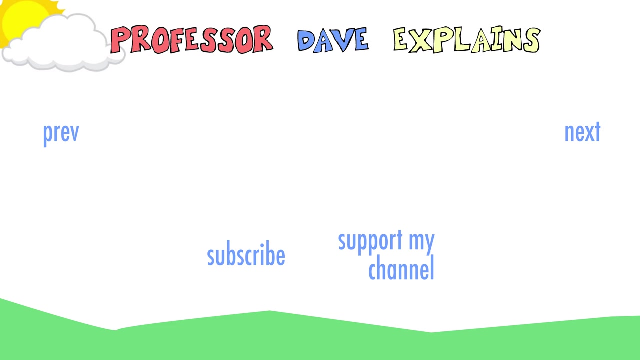 Thanks for watching guys. Subscribe to my channel for more tutorials. support me on Patreon so I can keep making content and, as always, feel free to email me professordaveexplains at gmail dot com. I'll see you next time. Bye-bye, Bye-bye.